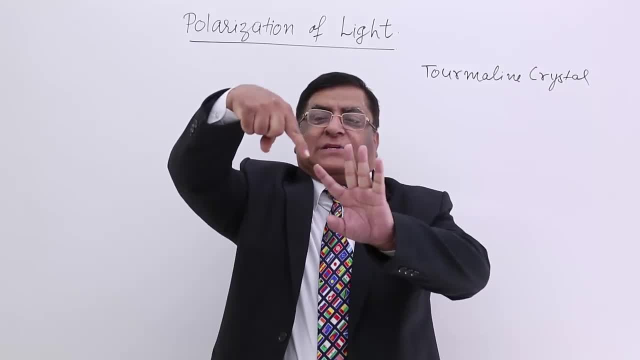 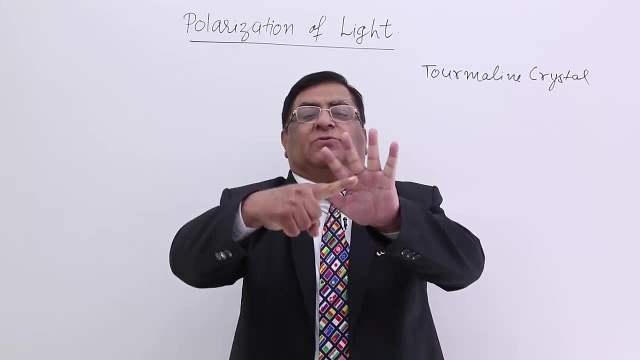 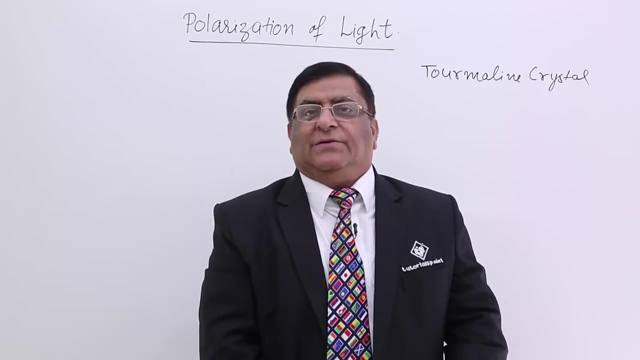 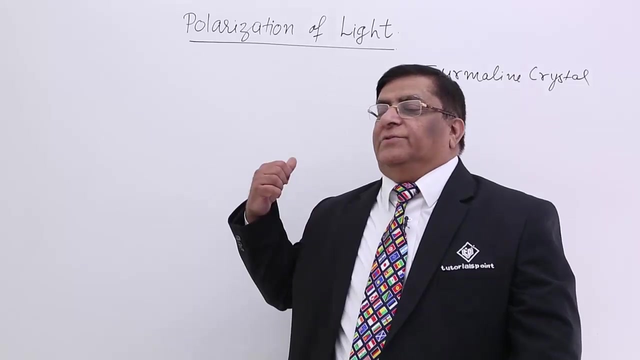 the opening. Anything of this size comes here, it can pass, But if something comes in this polarity, this will get stuck, It will not pass. This is something which comes to our mind and with that we searched and researched and found this theory of polarization. 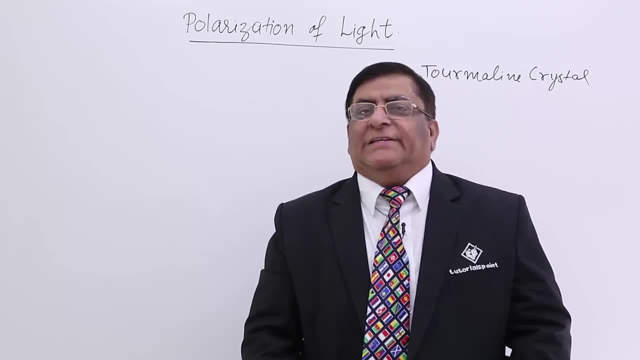 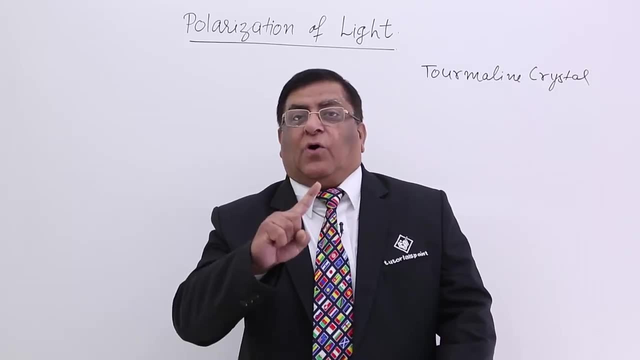 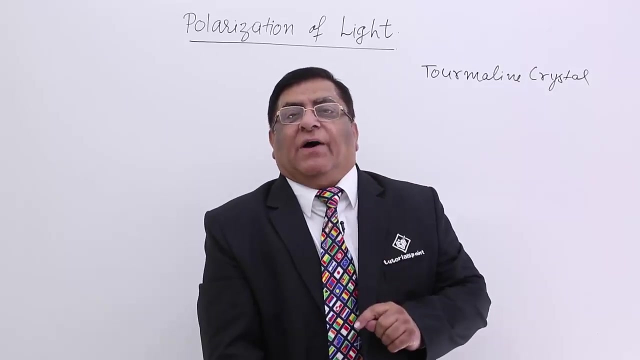 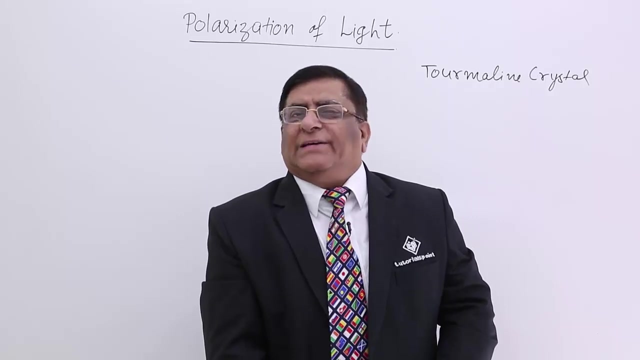 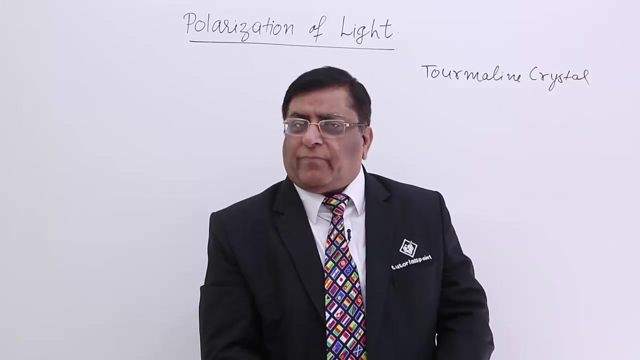 Now, what is this theory? This tells us that light is. light is form of wave, and the waves of light have a directions. The vibrations of light have a direction and they are polar. What does that mean? I tell you very clearly, very simply, how there can be a direction. The light is a particular 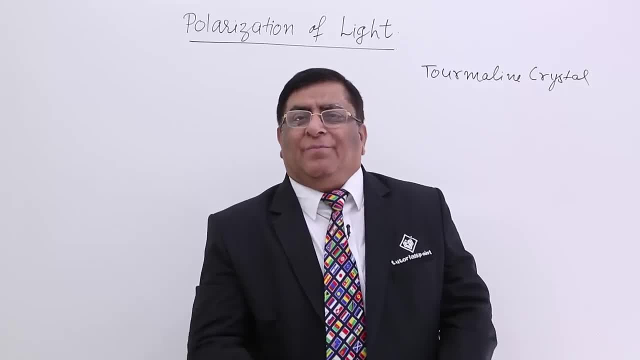 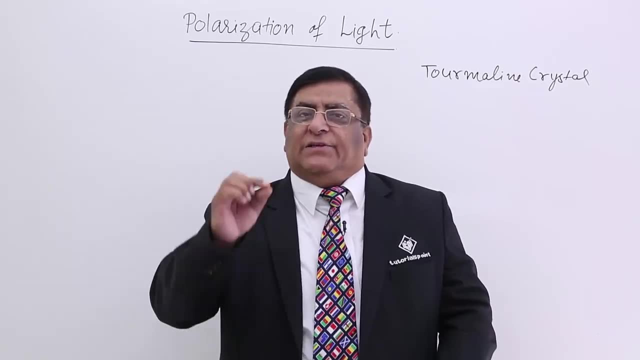 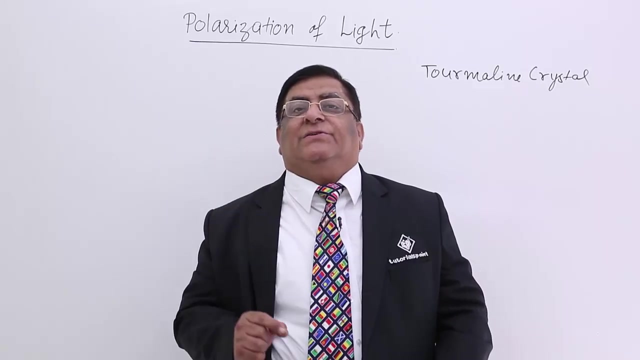 direction. The light is the form of the wave. This tells us that light is a form of wave generated by basic, by oscillation of electron inside an atom. when there is a oscillation of electrons, which is a accelerated motion that creates an electric field, and that electric 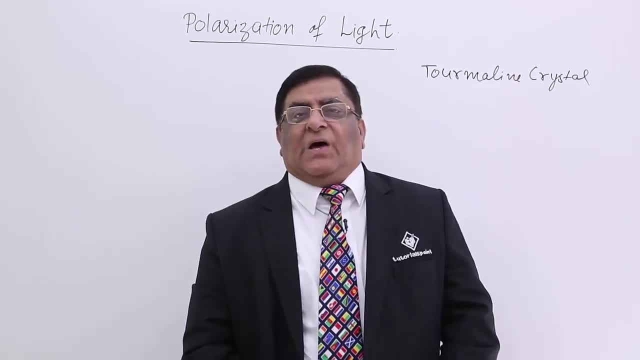 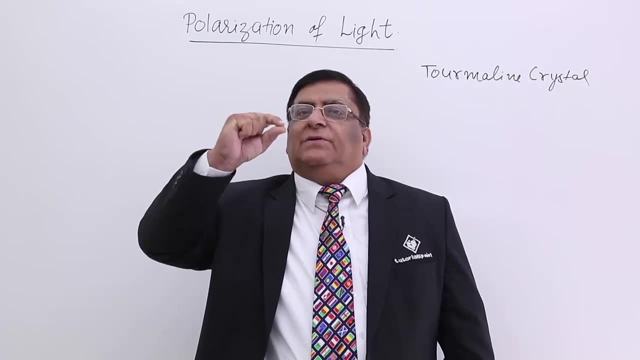 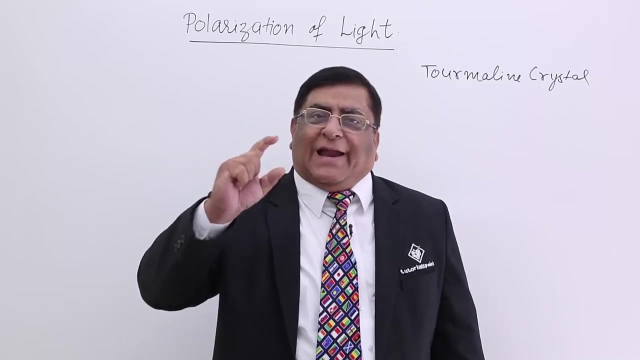 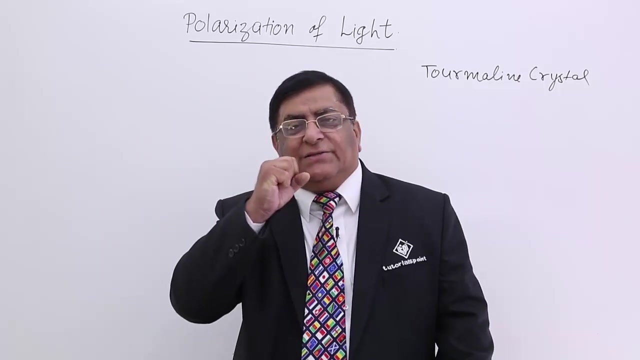 field we term as light. Now, an electron has oscillated this way, it has formed light, and that light carries the signal of that atom. it has come from that atom, and all that light of the material which comes to my eyes give me the image of that material. ok, 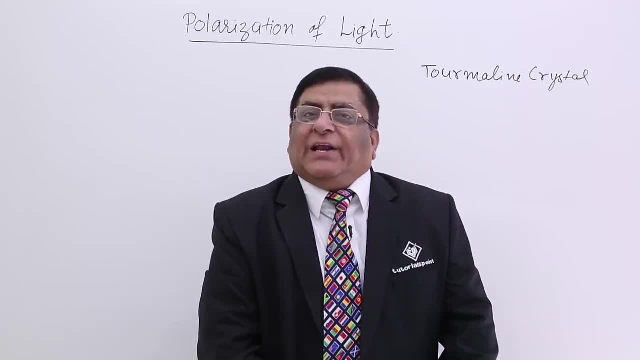 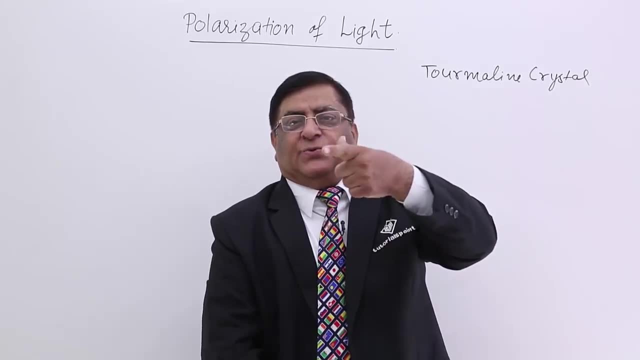 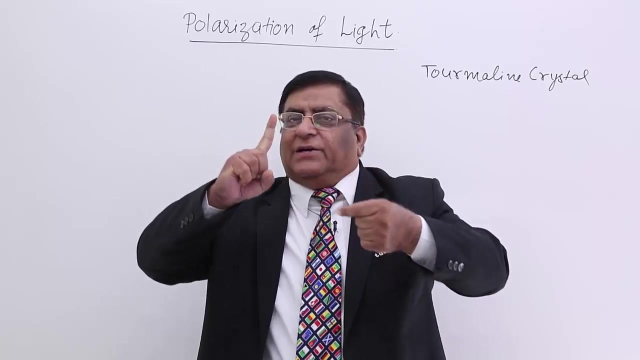 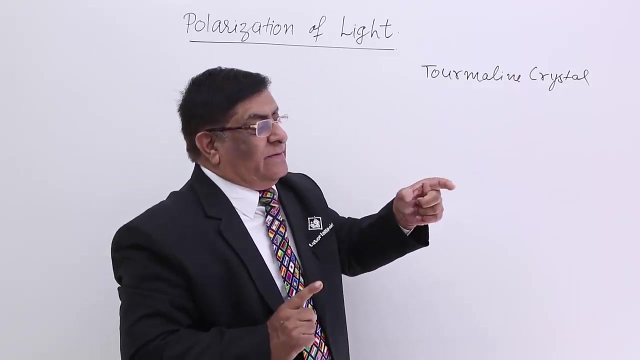 Ok, Now there is another electron that is also oscillating, but see, the direction of its oscillation is this way, This x, this was oscillating in this manner, so electric field was this way. It is oscillating this way, so its electric field is this: This has got electric field. 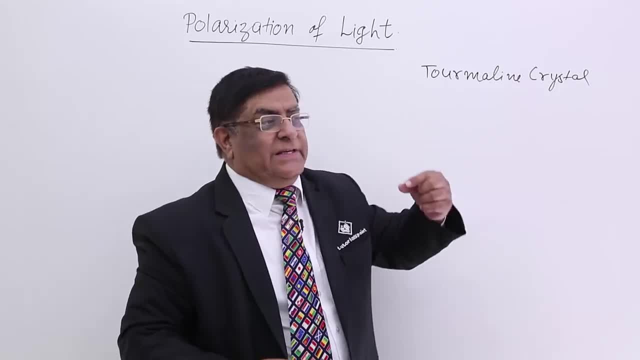 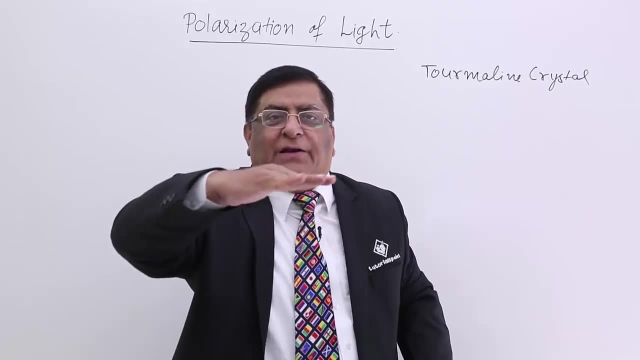 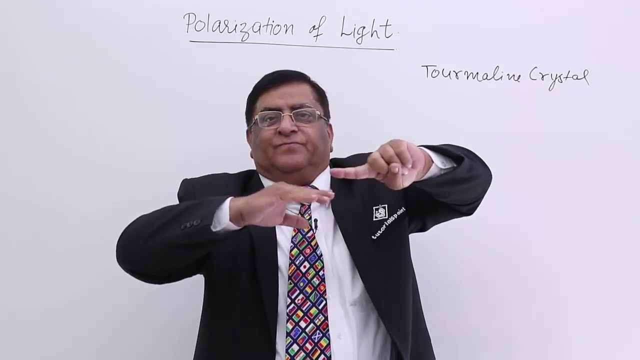 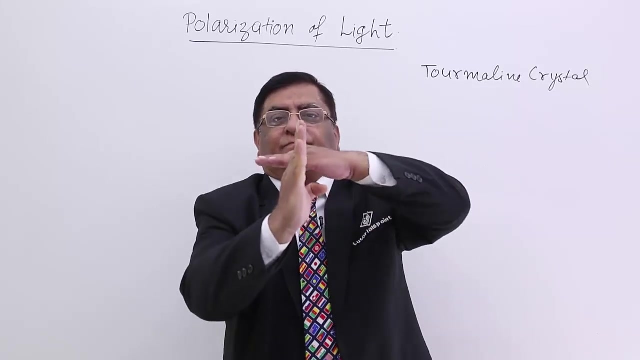 this way. It is coming to you. This has got electric field. this It is coming to you Now. this electric field has got a plane which has got two ends. its polling direction is this: This electric field is also polar and its direction of vibration is this: and these two are coming to you. Are 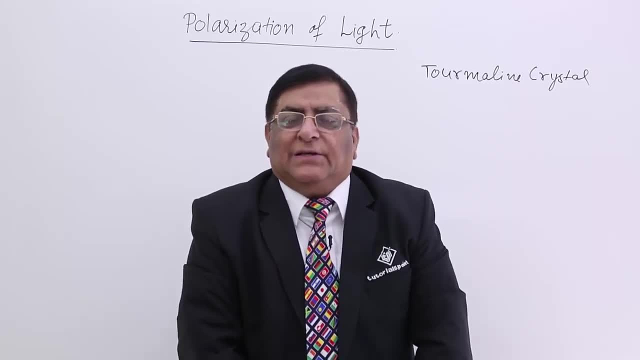 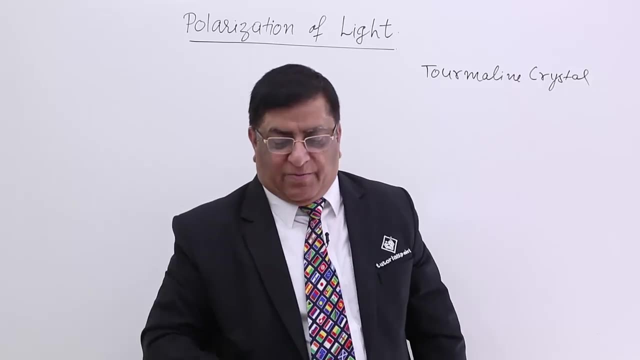 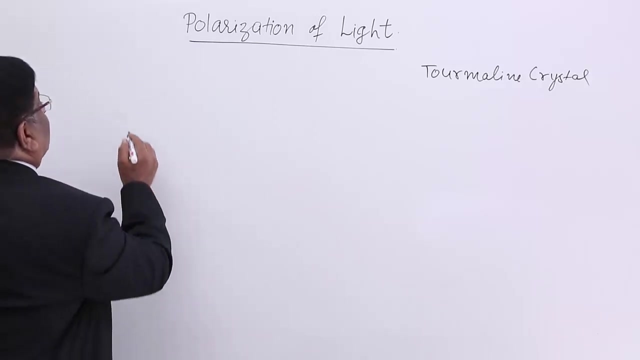 there only two? Answer: no, There are millions. Some electrons are oscillating this way and this is their vibration, Some this way, their vibration. So if a light is coming to you, I would like to express it here. It has certain vibrations in this direction, certain vibrations in this direction, some. 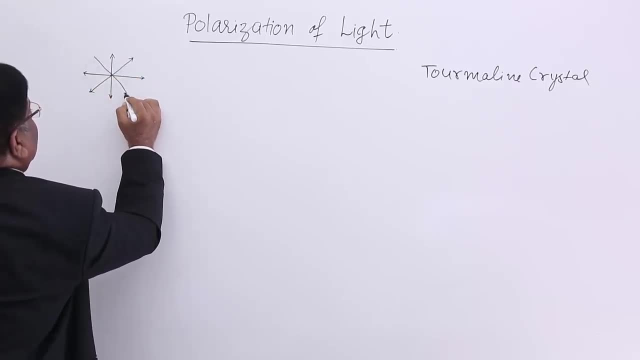 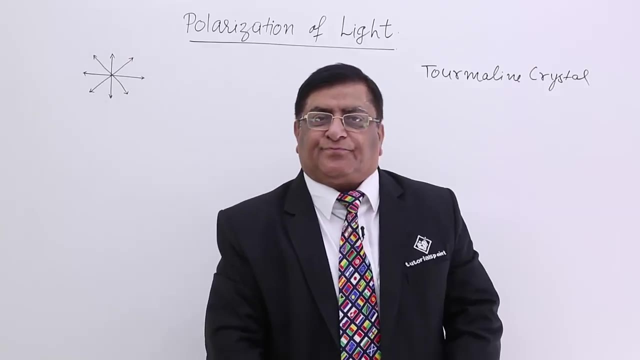 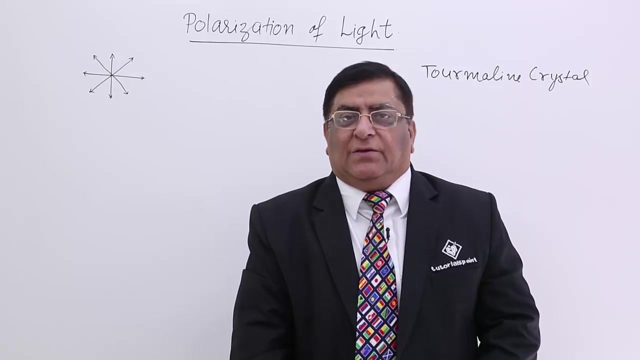 in this direction and some in this direction. That means some of these electrons are oscillating these all the directions. it has got vibrations and it is coming to you. This is the light, and whatever small quantity of this light comes to me, I am able to form the image of. 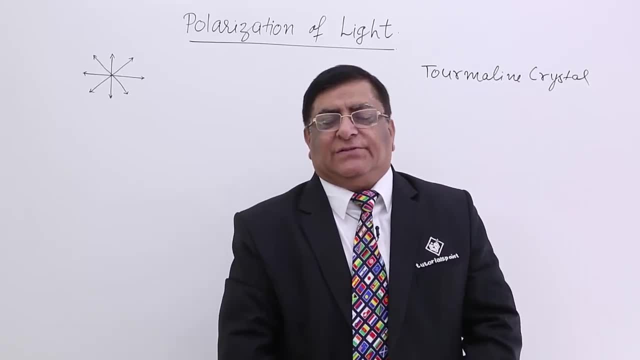 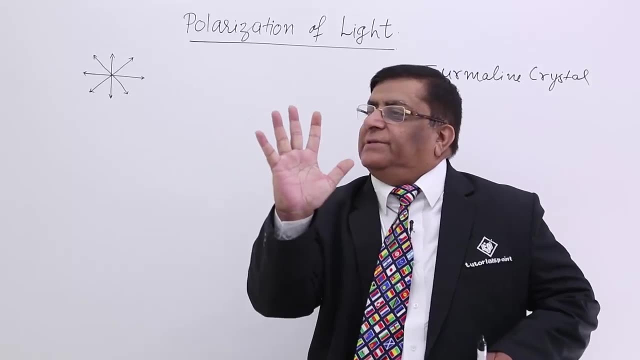 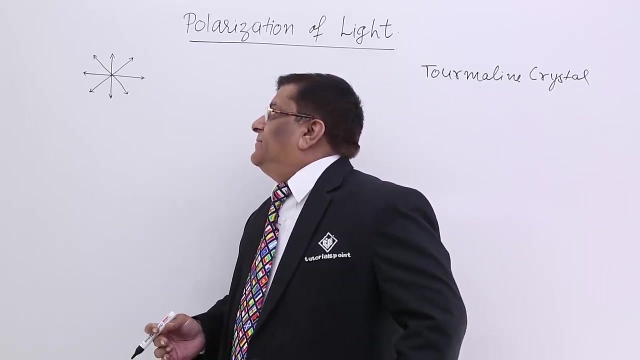 the source of this light. That is how we see the things. okay, Now this light is coming to you like this: Now, if I make a light, if I make a light, if I make a light, if I make a side way, then the side picture will appear like this: It is coming this way. Now I make. 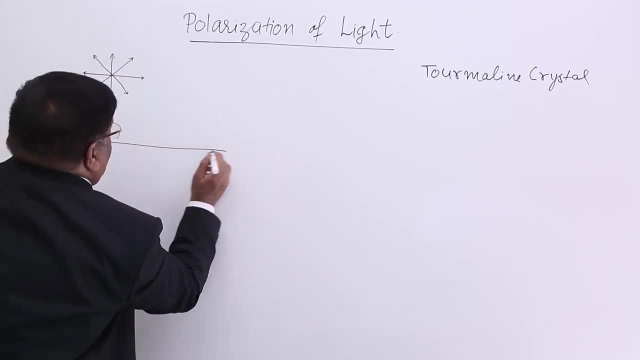 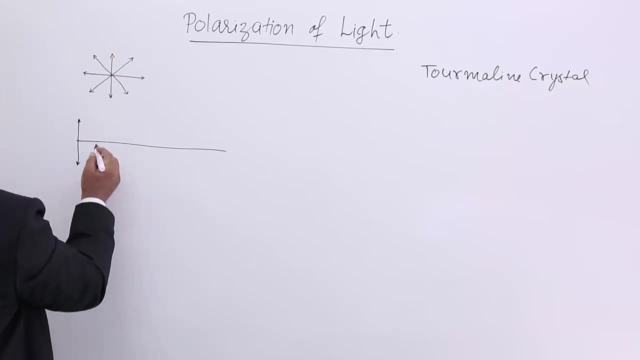 a side picture this way: Here there are these vibrations represented by this arrow and there are these vibrations I represent by a dot. This dot means this vibration, This means this vibration. So this light has vibration in both the directions and rest of the directions are included Then. 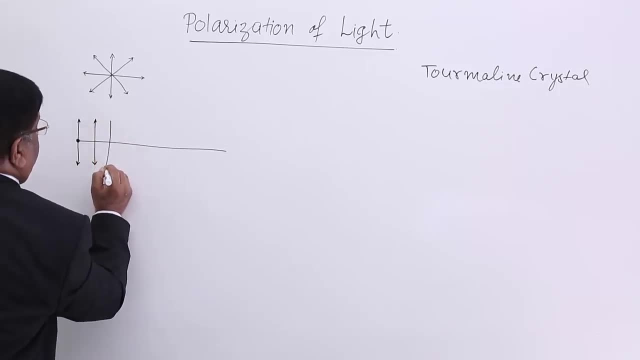 it is here And this light is moving in this direction. this is in this direction. this is front view and this is side view. Here is the velocity and here is y section, z section, y section, z section, and here is the velocity. This is we represent this light. Now, this light is. 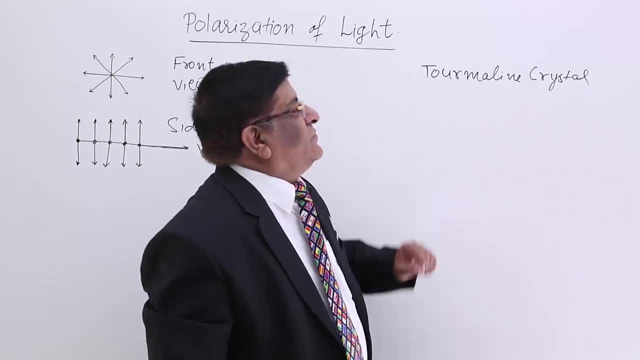 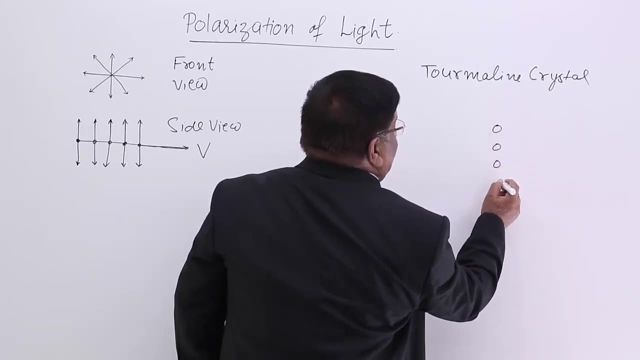 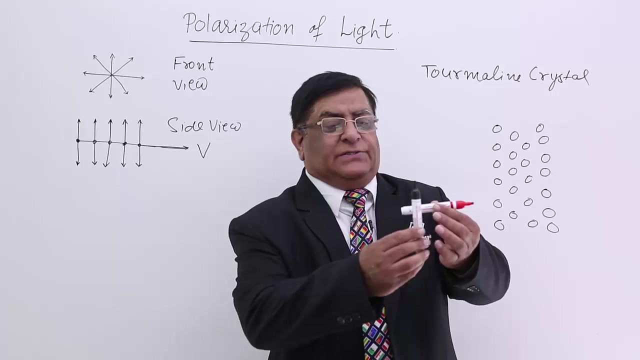 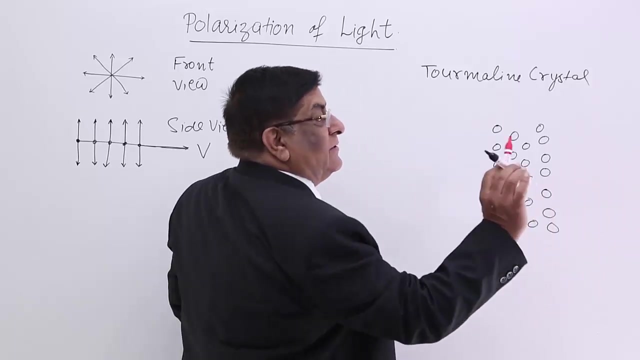 transmitted through tourmaline section. Tourmaline crystal has got molecules set this way. Now when the light comes here, the light has got vibrations in all the directions. Let us say these are the two main directions and the light is incident in this way. When the light 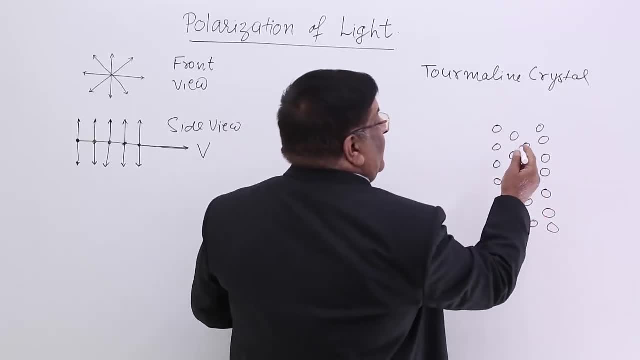 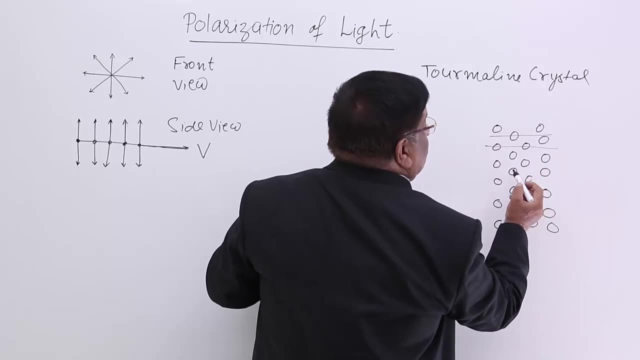 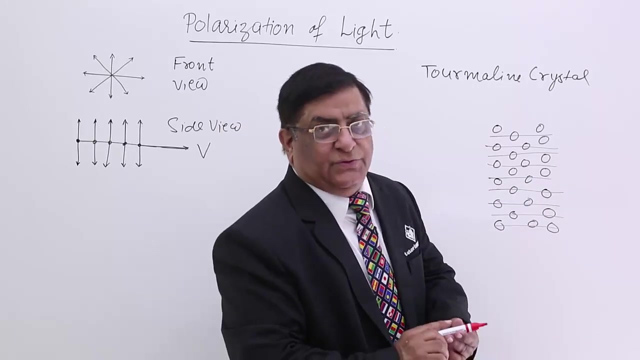 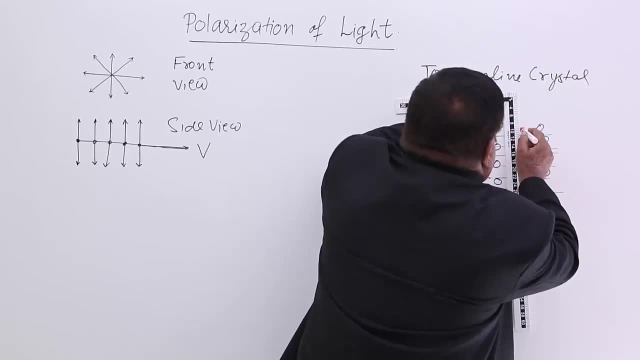 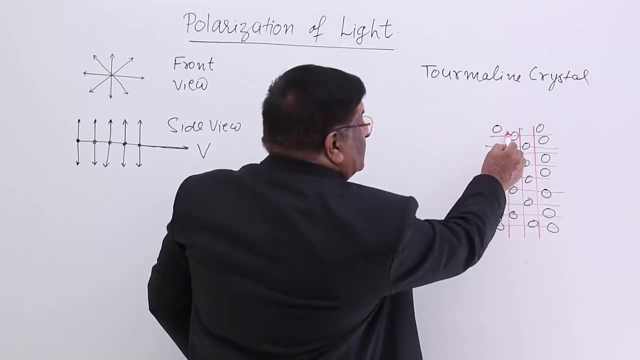 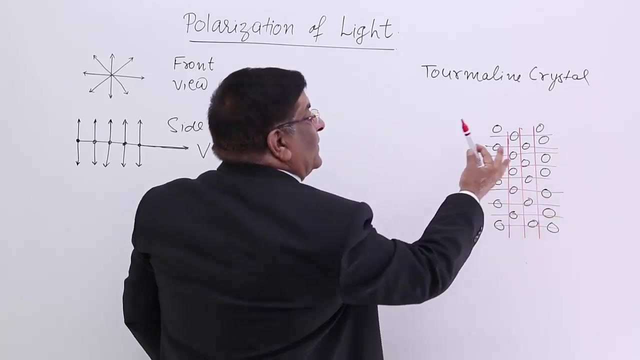 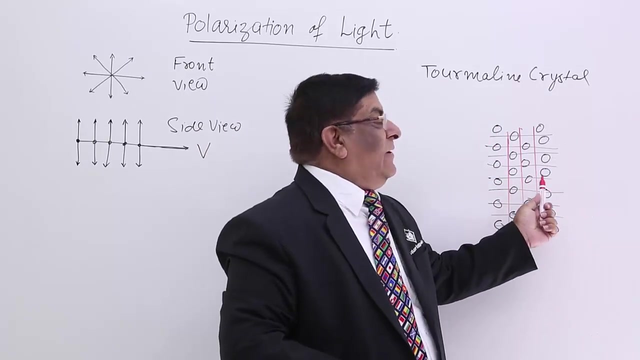 here and here and here a毫 Unterstütves- Without striking any molecule. without striking any molecule has passed Without striking any molecule. that means all the vibrations which are in this direction will pass through the tourmaline crystal and all the vibrations which are in this direction will pass will. 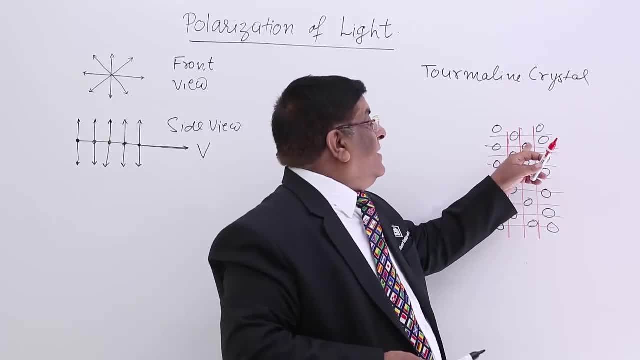 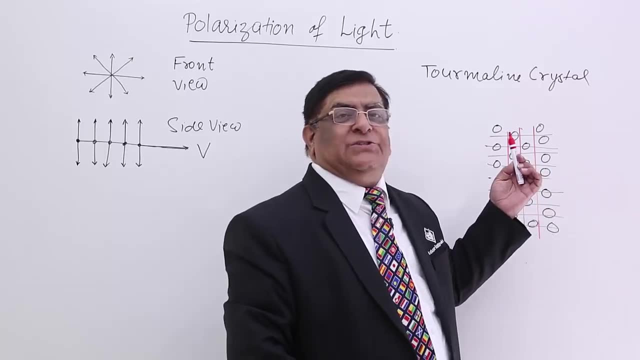 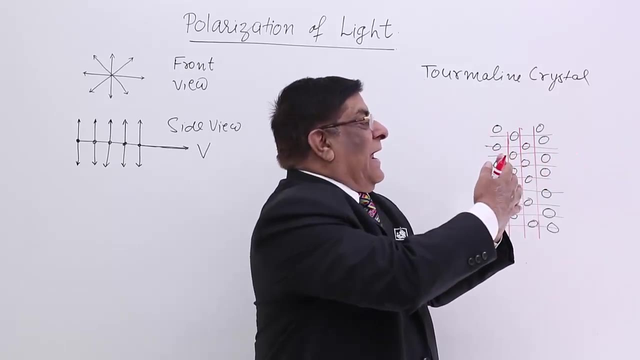 not pass through this, they will be absorbed by either of the molecules everywhere. So when it pass through, after that what happens? This is the turbulent crystal. from there the light is coming and half of the vibrations have been absorbed and half are coming to my eyes. 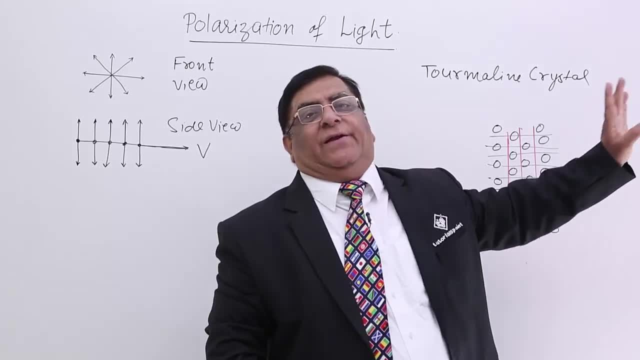 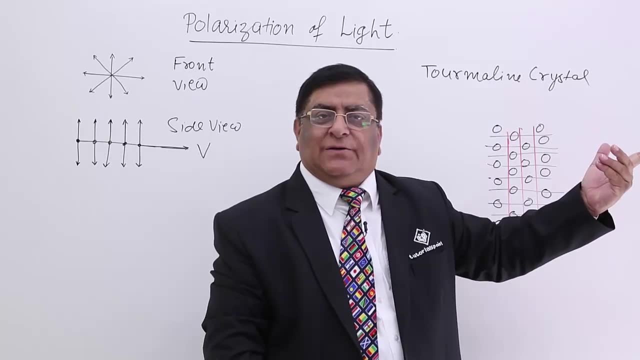 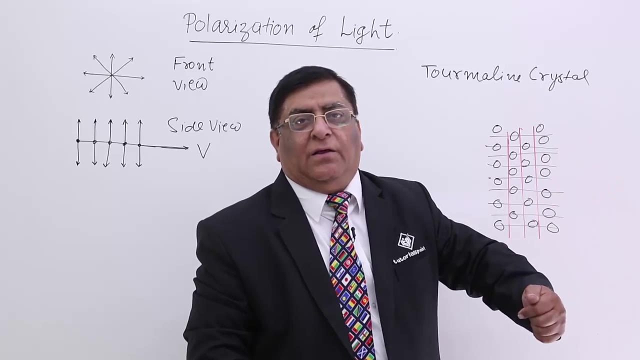 What do I see? Answer: I see the same thing. what is there? If I am seeing a chair without any crystal, I put a crystal here. I see the same chair. What is the difference? Answer: the difference is: earlier, without crystal, if 100 waves were coming, 100 waves were coming. 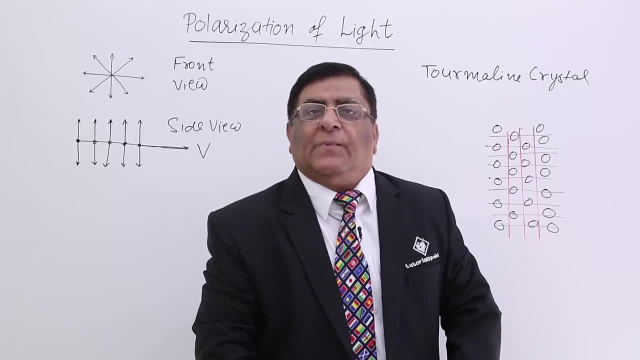 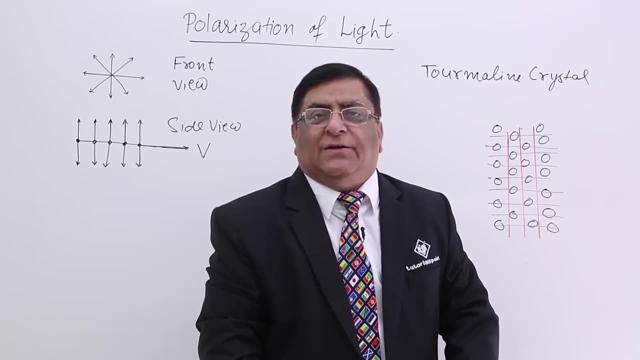 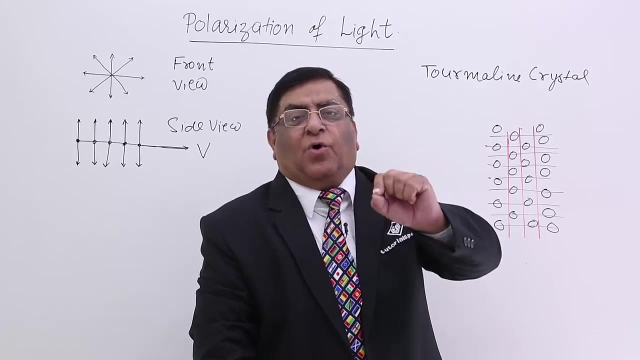 now the waves coming are 50. Does it make in the image of chair? Does it make any difference to the image of chair? Answer: no details. there is no difference because a very small number of waves coming from the chair will form the image and I will be able to see the chair. 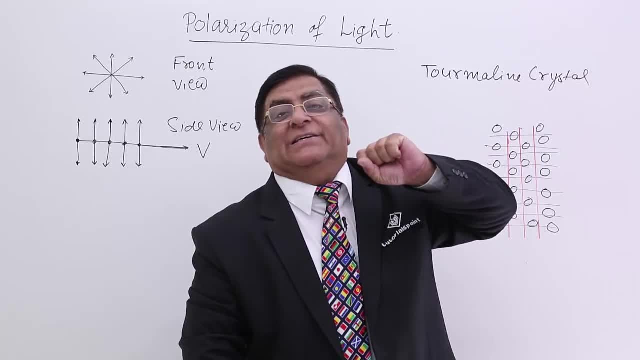 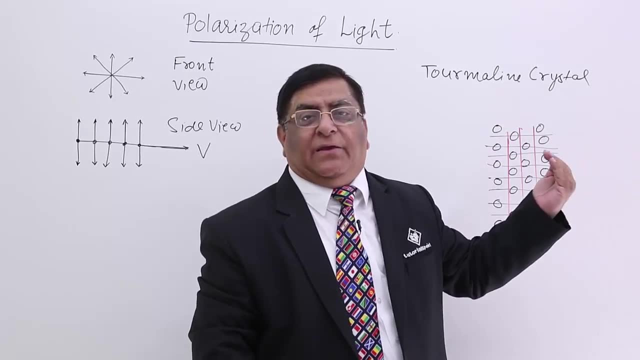 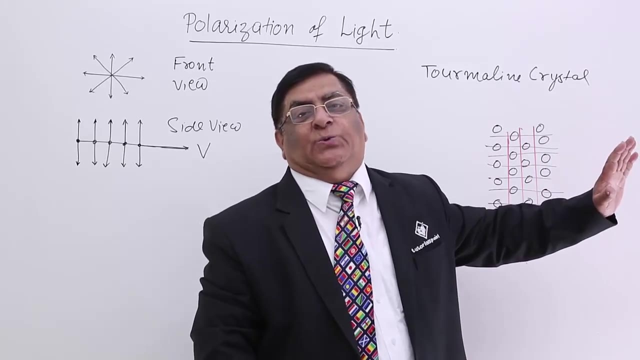 Then what is the difference? The difference is in the intensity, in the brightness. The 100 waves coming from the chair make it very bright. The 50 waves coming from the chair make it less bright, as if the chair has been put in a shadow. 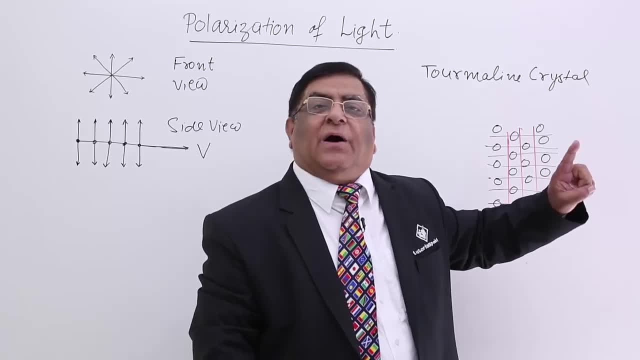 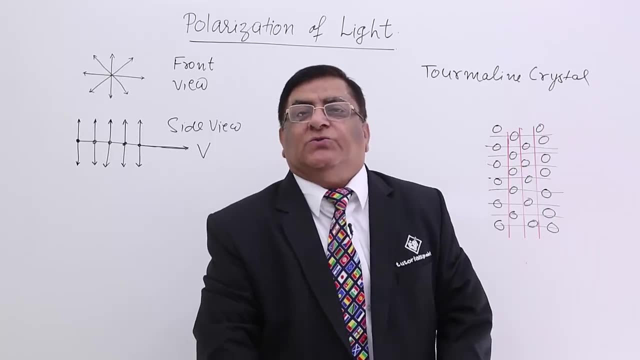 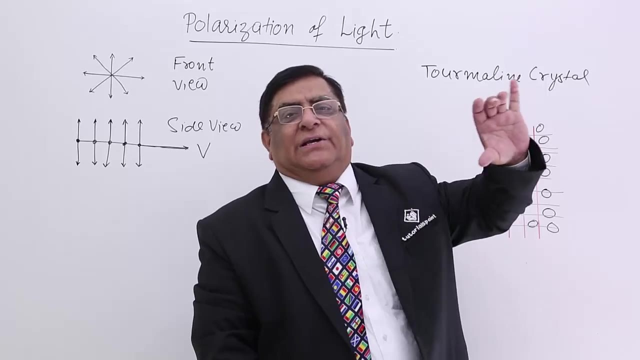 So without rodent crystal, it appears as if it is in the sun. with crystal, it appears as if it is in the shadow. So what has decreased? Answer: intensity has decreased. and what is intensity? you know, it is energy per unit time, per unit area. 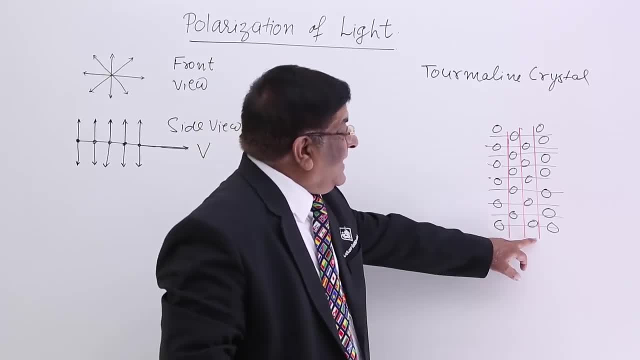 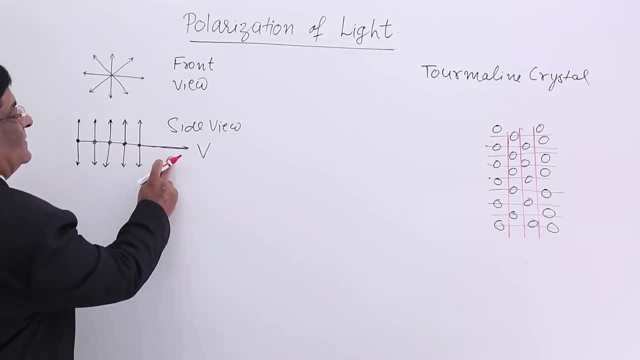 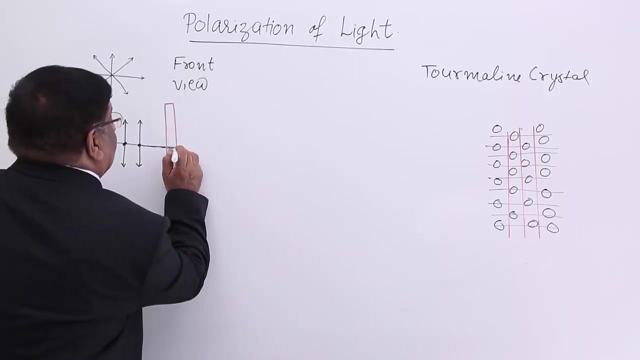 So now this light is coming to me, This I represent here, This is the light original, and here I put a crystal. Now, when I put the crystal here, what is the shape of the light here? Now I get this, This thing, This vector. 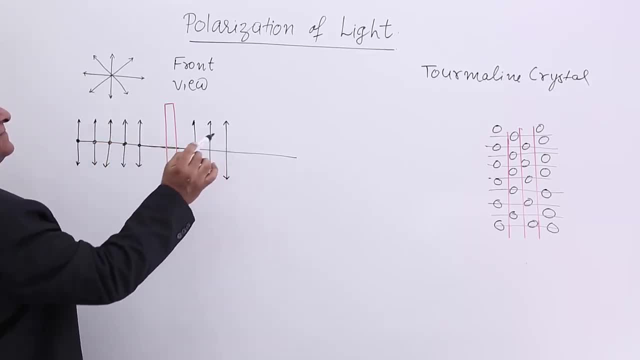 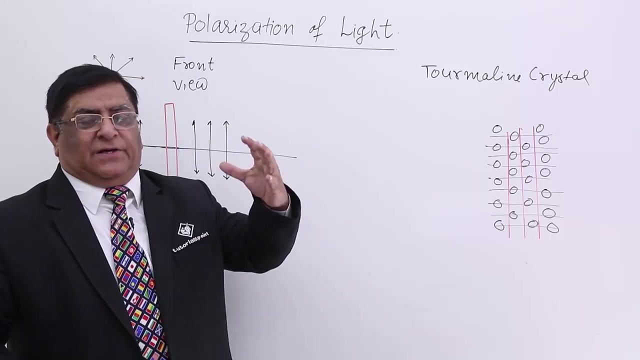 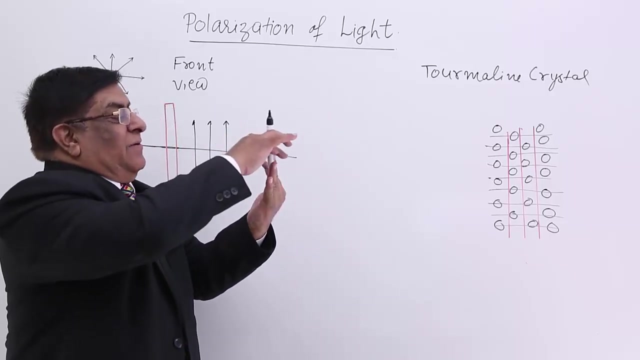 Of the light is missing. this is this vector has passed through because it was having this crystal is having all the windows set in this direction. I cannot make it out- there are different methods to make it out- but say if all are in this direction, then these are the vibrations which will come out. 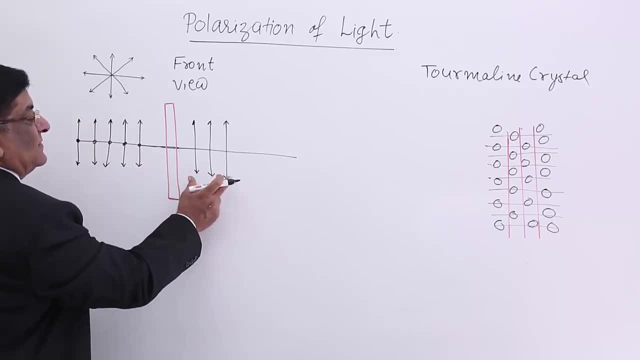 This light and this light. What is the difference? There is a difference. So this will be the light and this is the termini. love And these are the samecriptions. The brightness will be less If I see the object in this light. 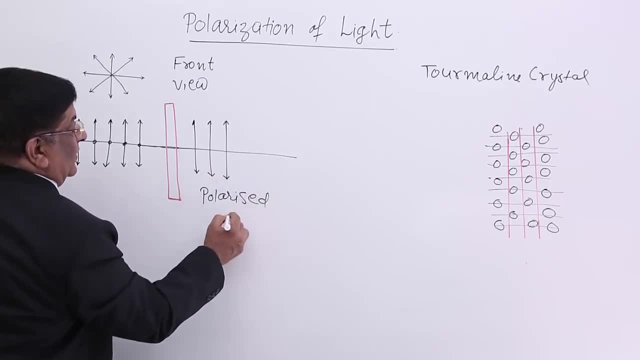 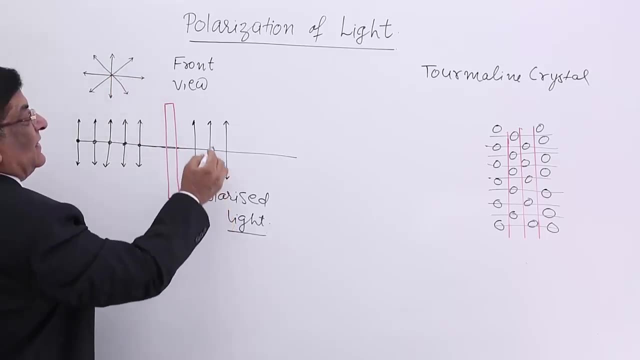 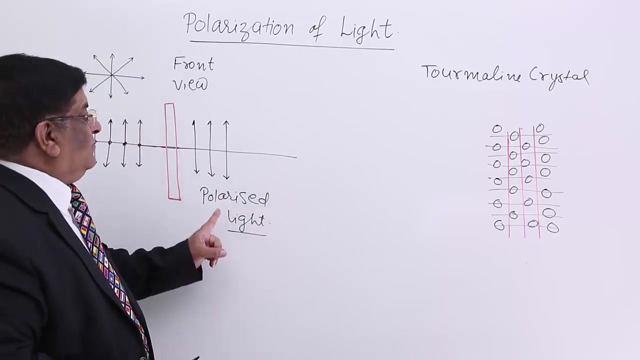 Now, physically, there is a change in the name. this I will call polarized light. polarized light Why? because here it has got all the directions, Here they have one direction. Once they attain one direction, We say they have become polarized. of that, This is polarization of light. okay, Now if this light is polarized or not polarized? 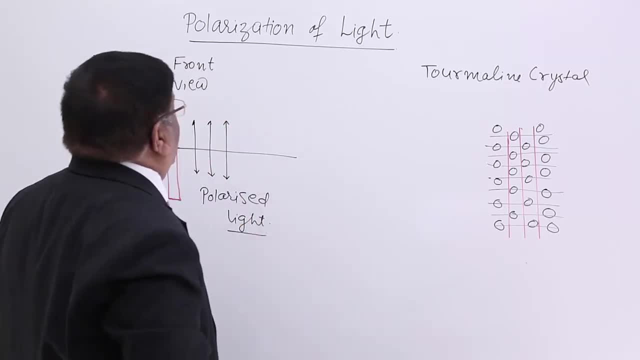 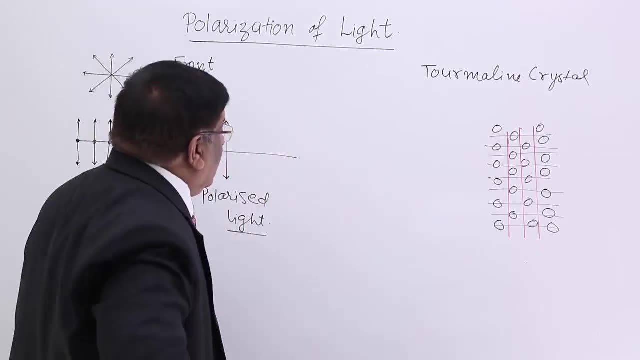 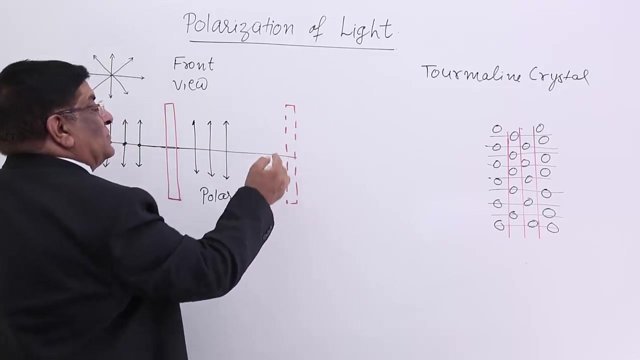 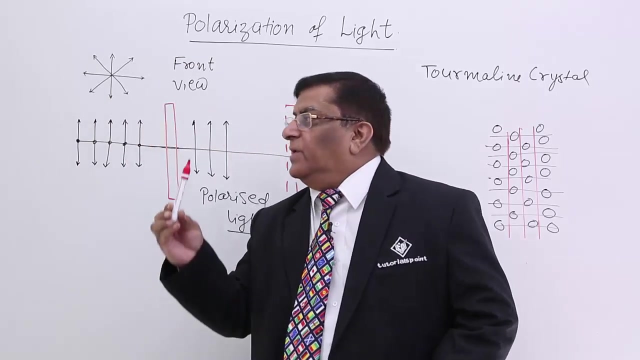 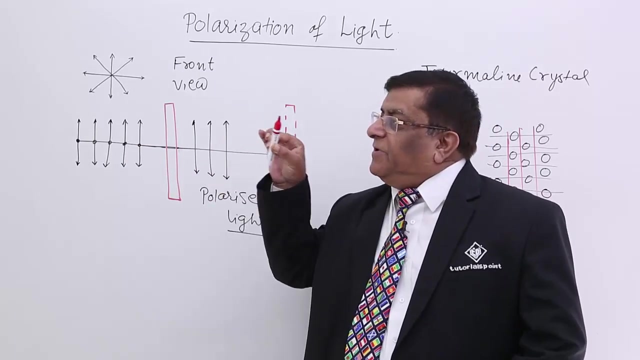 how do I know, Then, what I do? I put another crystal here, another crystal here. Now this crystal has also windows in a certain directions. I do not know what direction, but one thing I know: I start rotating it, I find at one position it is giving me the full view, as. 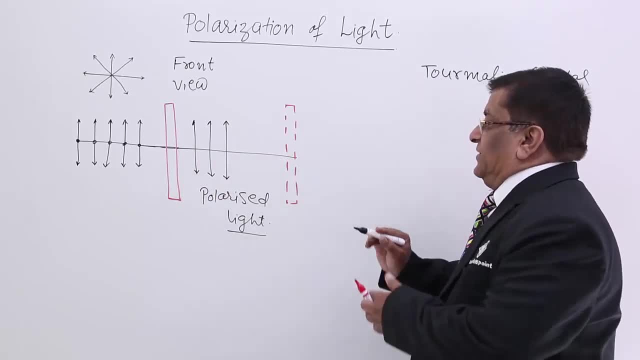 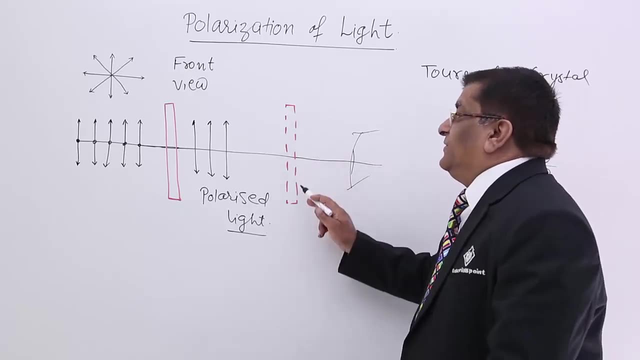 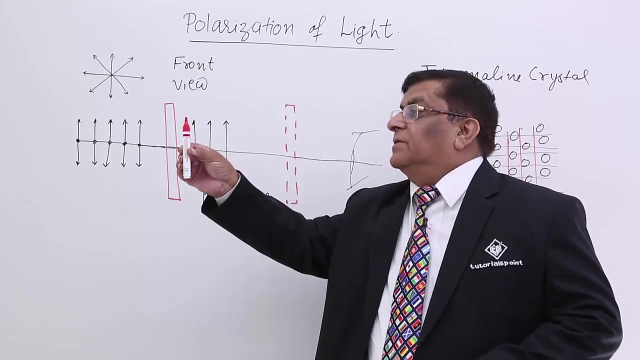 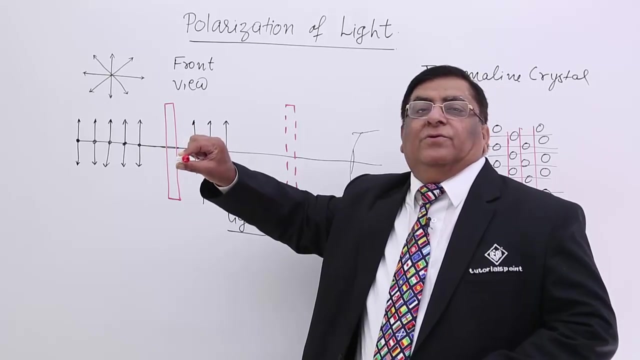 without this, with this- I am seeing it here, I am observing it here. Without this, I am seeing it here, Without this: there is certain brightness With this. the brightness, yes, same brightness. now the brightness has decreased. now it has decreased. now it is no more there. 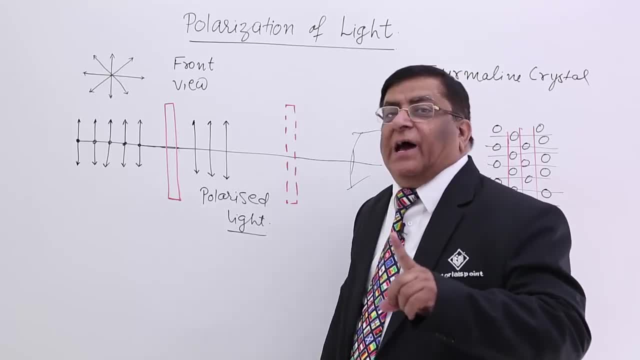 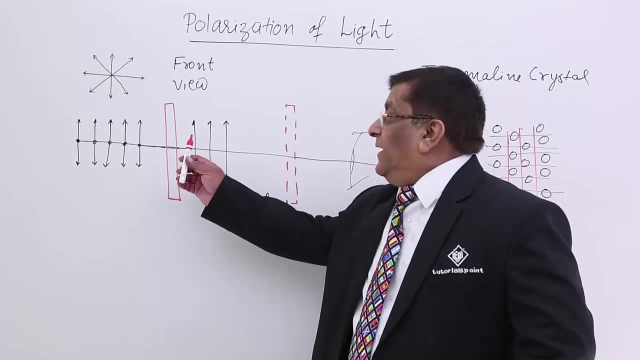 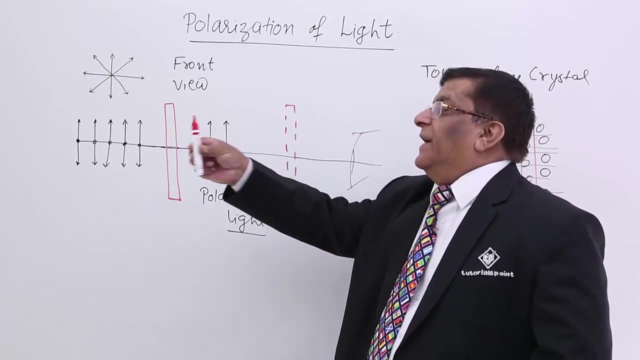 If it happens, if it happens, I will declare that this was polarized light. If this does not happen, like in this case, If I rotate this, if I am keeping it, this, this vibration is coming. I see the chair. 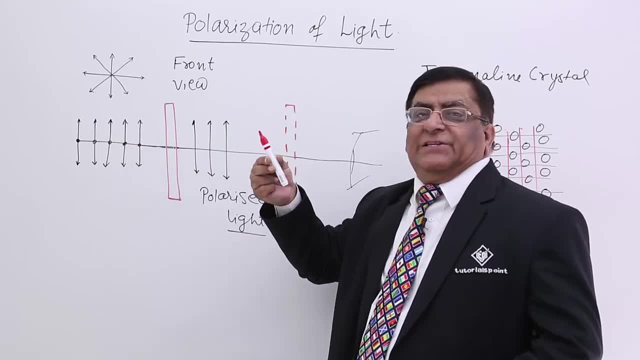 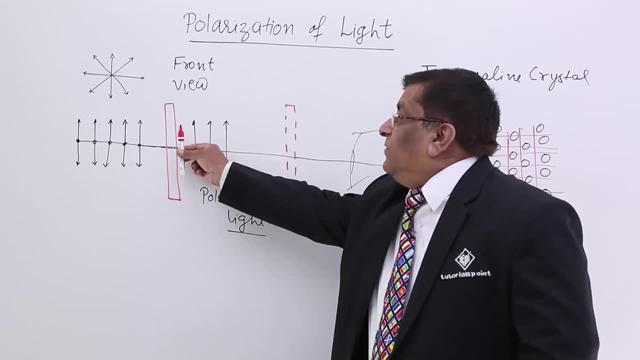 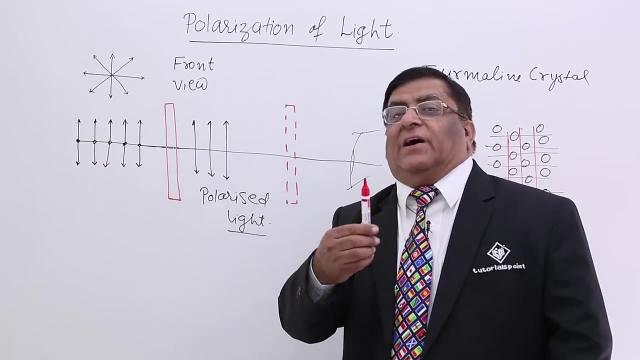 If I rotate it this way, this vibration is coming. I see the chair. If I rotate it this way, this vibration is coming, I see the chair. So, in whatever direction I rotate it, I see the chair. So I will declare that the light which is coming is unpolarized. 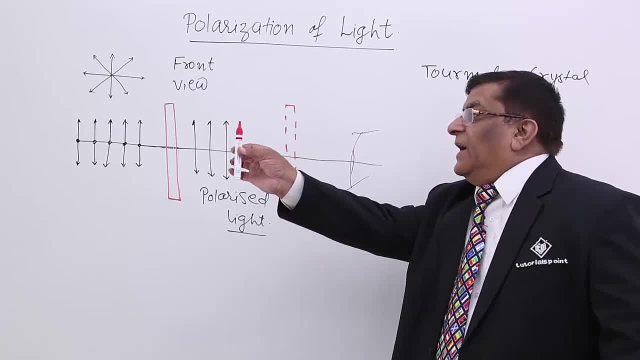 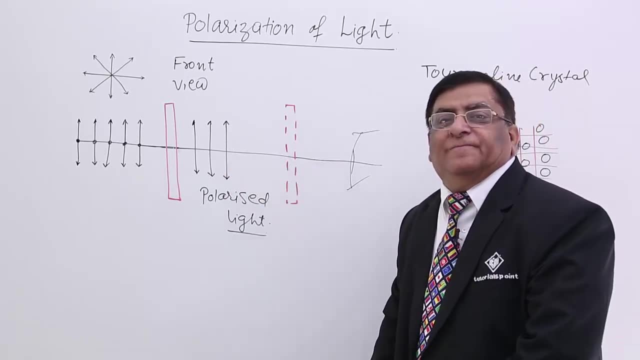 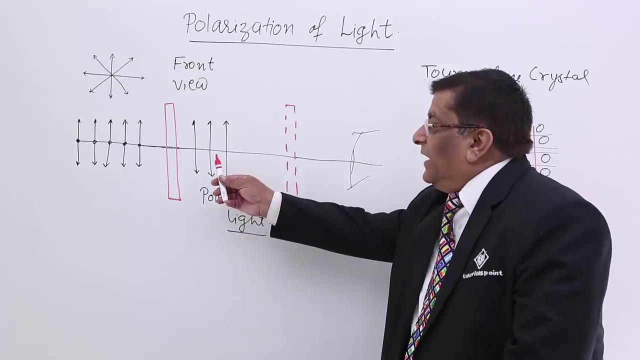 But in this case, when I rotate it, I see the chair in one direction, but when I turn it by 90 degree, then I don't see the chair. It just become blank nothing. So then I declare the light which was coming was polarized. 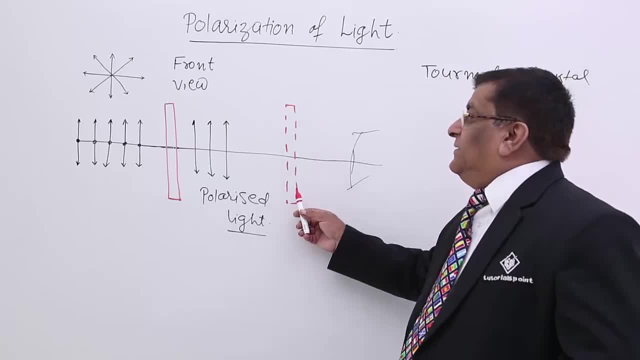 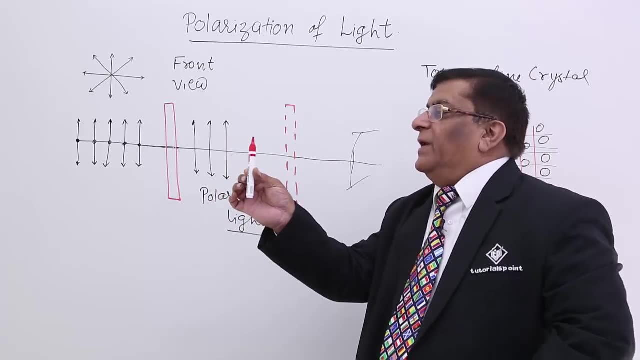 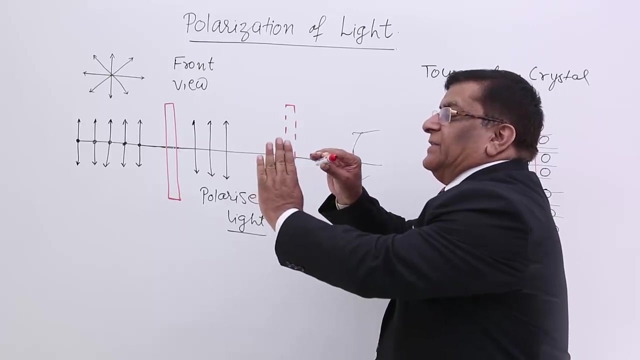 Because this polarizer, this crystal, has window only in one direction That will show me the chair when the waves coming are having this direction of vibration. And if I turn it this way then light does not come to me and I see darkness there. 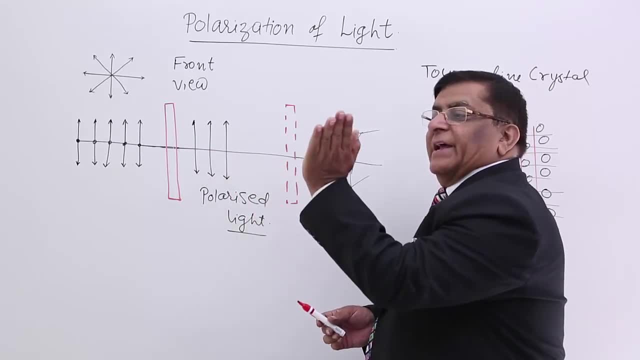 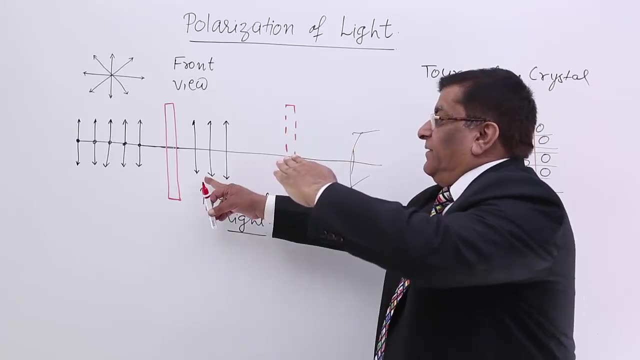 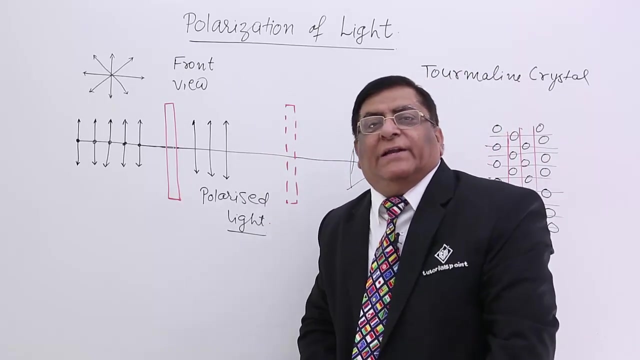 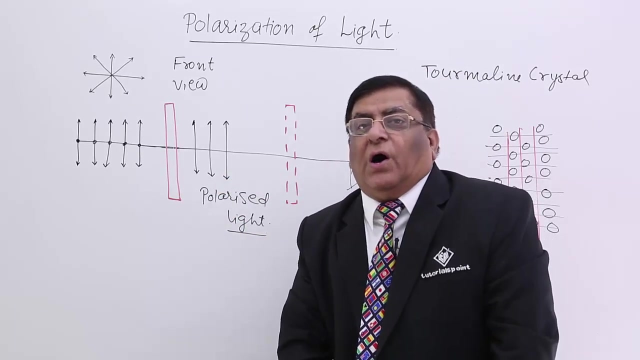 Suppose these are coming in this direction. so when I put it this way, I see full bright chair, whatever is the brightness here, and when I rotate it 90 degree I see it is surround dark. What does that prove? That prove that this light is a polarized light. So how do 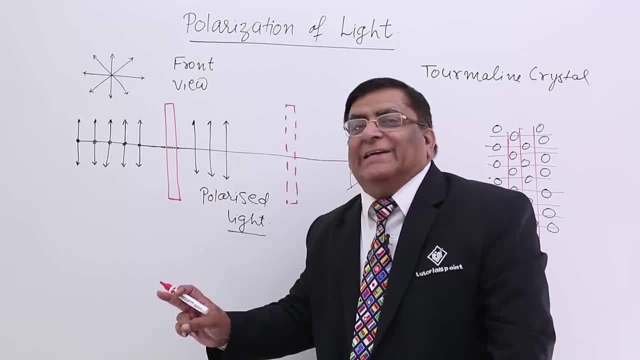 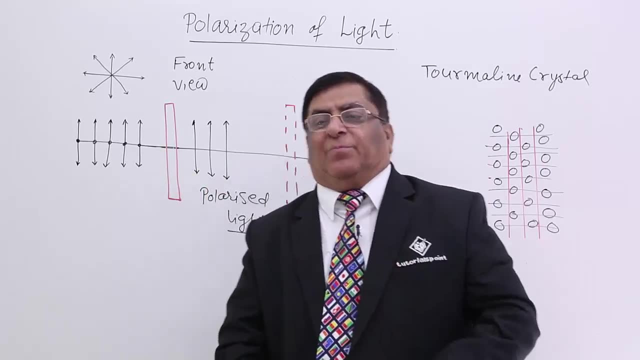 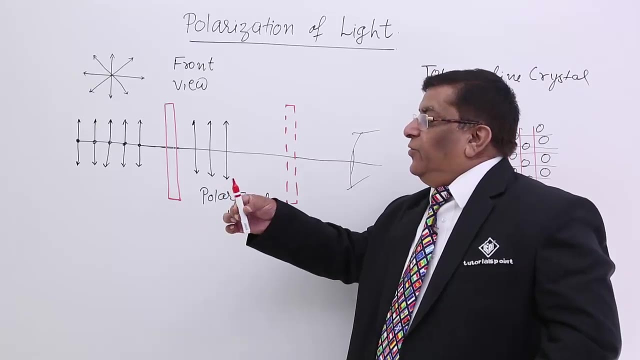 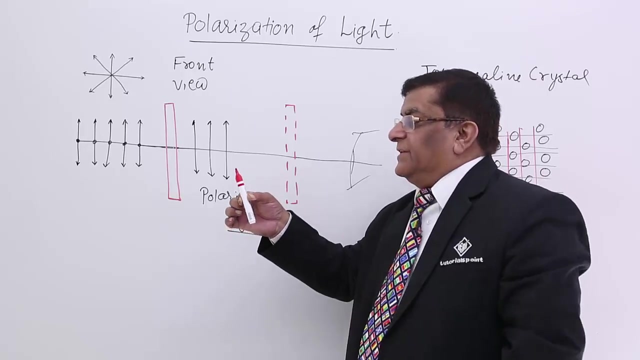 we know whether a light is polarized or it is not polarized? The answer is: with the eyes. we cannot make it. We need help of this crystal and we have to keep this here and rotate it. See the object through this. If I am seeing the object with certain brightness change. 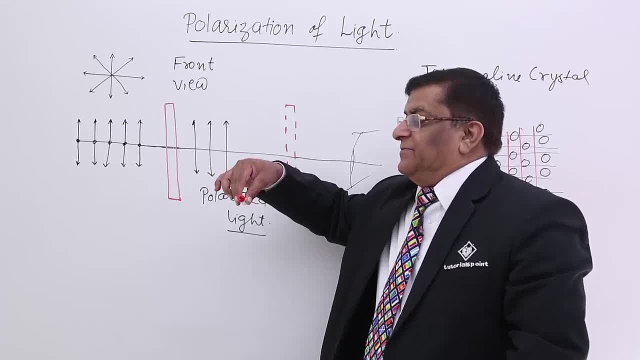 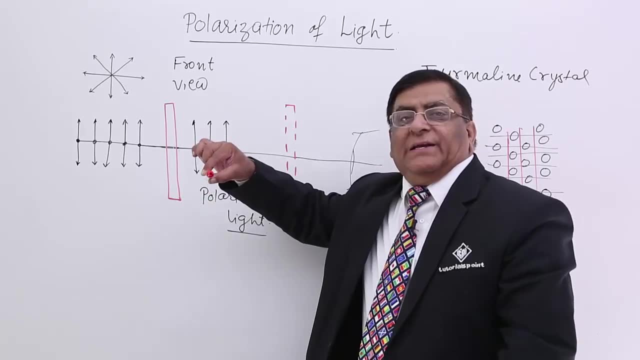 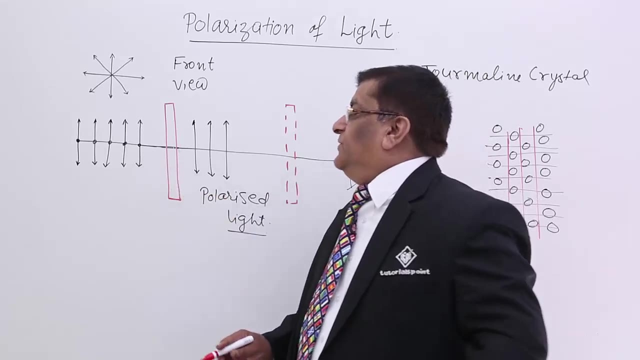 in brightness, change in brightness, brightness finished, then I will say the light is polarized. If same brightness, same brightness, same brightness, then I will say that light is unpolarized, non-polarized, So this light is unpolarized. 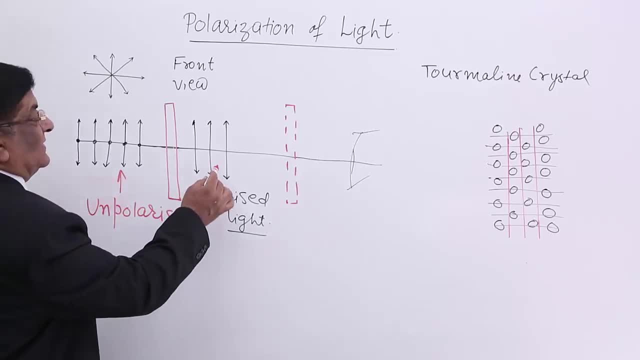 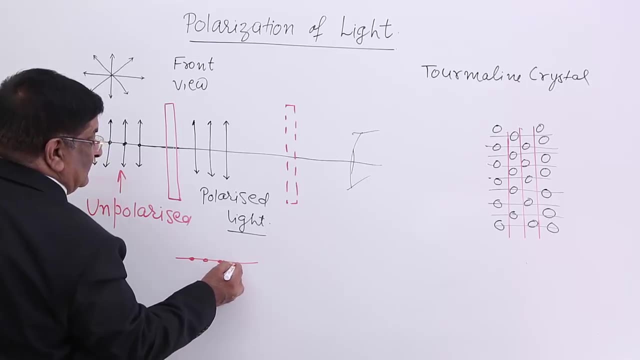 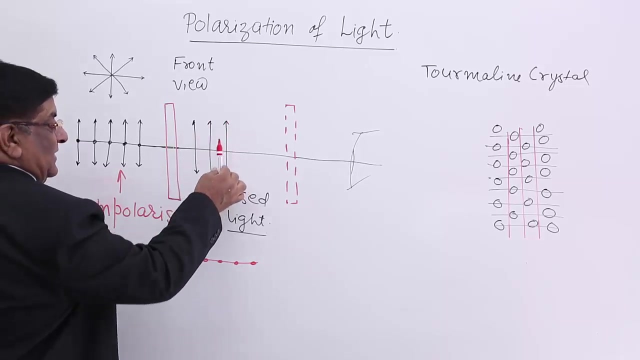 This is unpolarized light and this is polarized light. This polarized may be like this, or this may be like this. This shows that these vibrations are in one direction. This shows that these vibrations are in this direction, So it may be either this or this either.